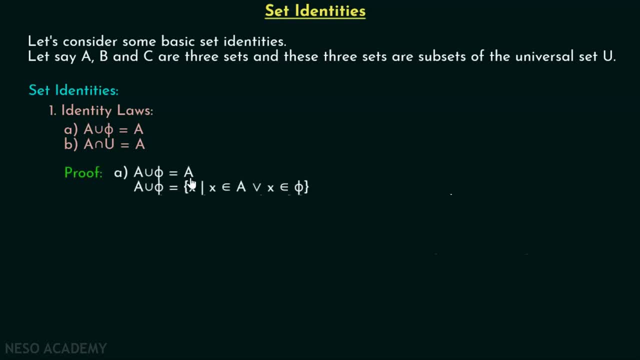 First we will prove that A union phi is actually equal to A. For this we know that A union phi is nothing but a set of all x, such that x belongs to A or x belongs to phi, Right? So either x belongs to A or x belongs to phi, or it can belong to both, Right? 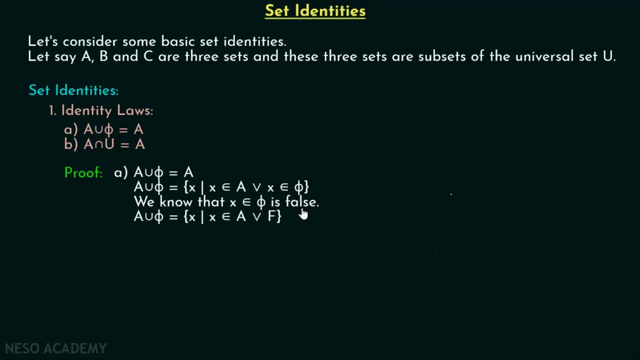 We know that x belongs to phi is actually false because there is no element that can be a member of phi Right, Because phi is an empty set. So here we know that x belongs to phi is actually false. So can we replace this x belongs to phi by f. 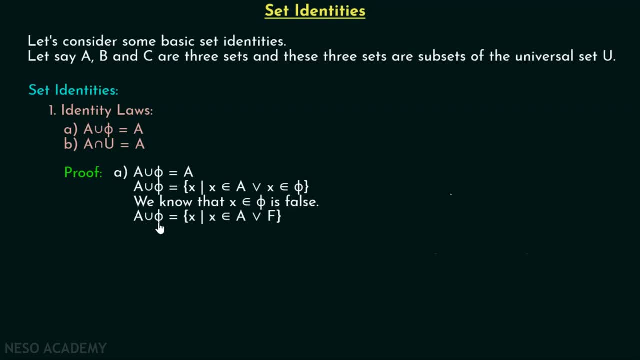 Yes, of course we can do this Right. Therefore, A union phi is nothing but a set of all x, such that x belongs to A or false or capital F. I am denoting false by capital F. Okay, Here we can replace this x belongs to A or f by x belongs to A, Isn't that so? 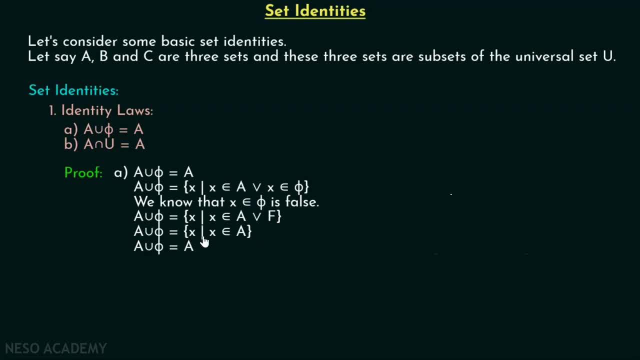 So this is how it looks like. So we have a set of all x such that x belongs to A. What does it represent? It represents set A. Please see this. We are talking about a set of all x such that x belongs to A. 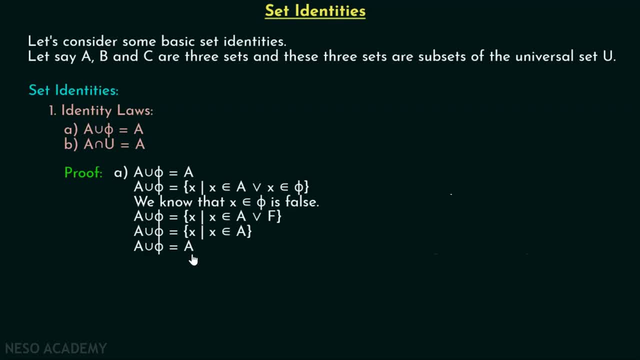 That means we are talking about set A. Therefore A union phi is nothing but A Right. Hence proved. Now let's try to prove second identity law, that is, A intersection universal set is equal to A. First we know that A intersection universal set is nothing but a set of all x, such that x belongs to A and x belongs to universal set. 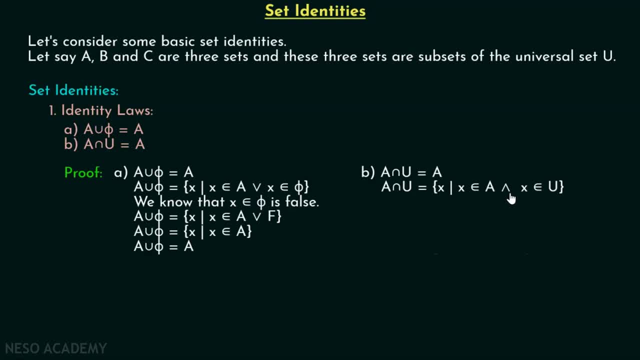 Here we are talking about intersection. Therefore- AND must come over here- x belongs to A and x belongs to universal set. That means x must belong to both of them, Right? We know that every element is contained in the universal set. U. 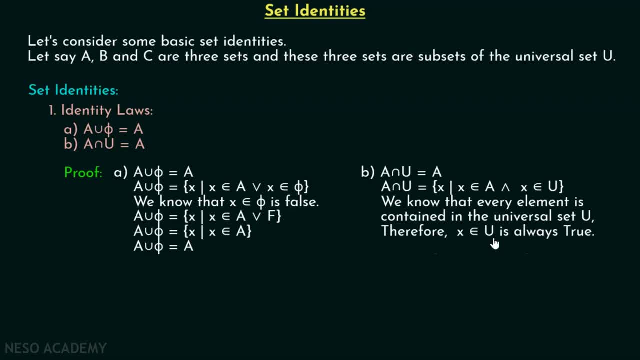 Isn't that so? Therefore, it is clear that x belongs to universal set is always true, Because there is no element which is outside universal set. Every element is within universal set. Thus, we can say that x belongs to universal set is always true. 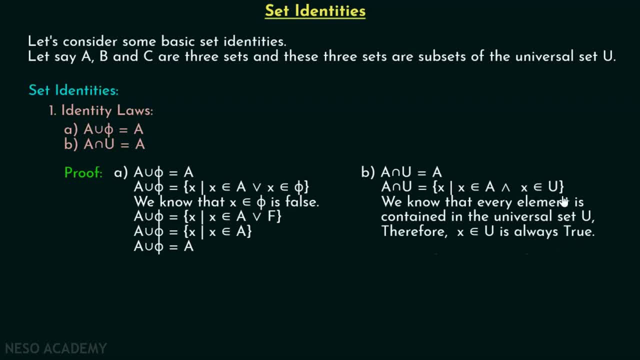 Isn't that so? Therefore, we can easily replace this statement, that is, x belongs to universal set, by true or capital T, And this is how it looks like A intersection: universal set is nothing but a set of all x, such that x belongs to A and true. 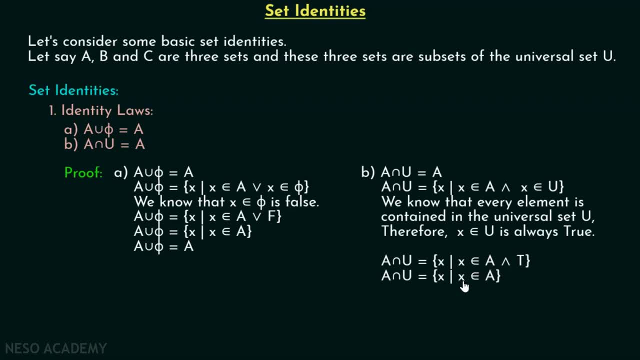 What is x belongs to A and with true, Obviously this is x belongs to A Right, So we can easily replace this by x belongs to A. A intersection universal set is nothing but a set of all x such that x belongs to A. 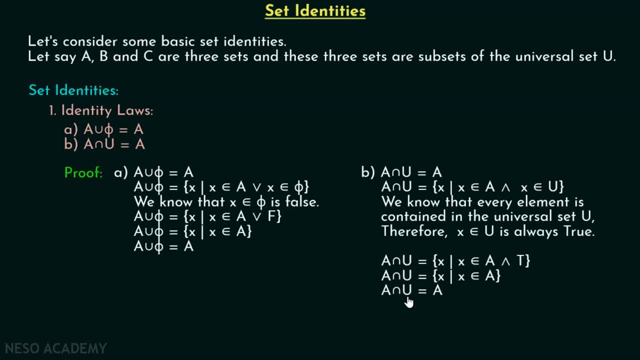 Or we can say that this is equal to A Right. Therefore, A intersection universal set is nothing but A Right. Now we will discuss our second set identity. that is A Second set identity, that is, domination laws. So there are basically two laws under this category. 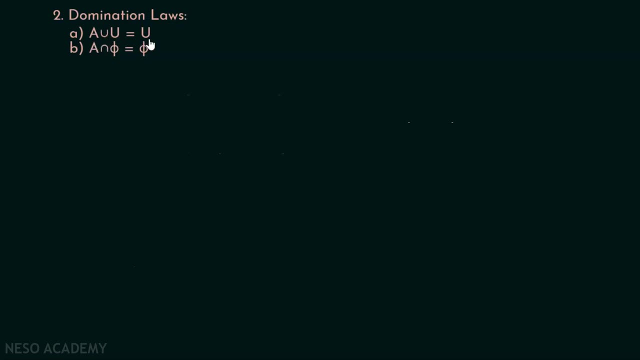 First is: A union universal set is nothing but universal set And A intersection phi is nothing but phi. Okay, Let's first discuss A union universal set equal to universal set. Here we know that A union universal set is nothing but a set of all x. 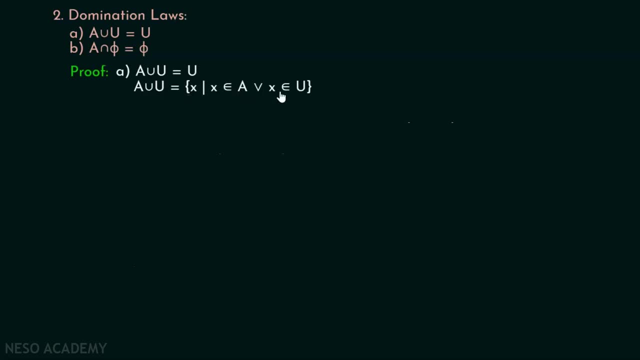 such that x belongs to A or x belongs to universal set, Right? Either x belongs to A or x belongs to universal set, or x belongs to both. This is what union is all about, Right? We know that x belongs to universal set is always true. 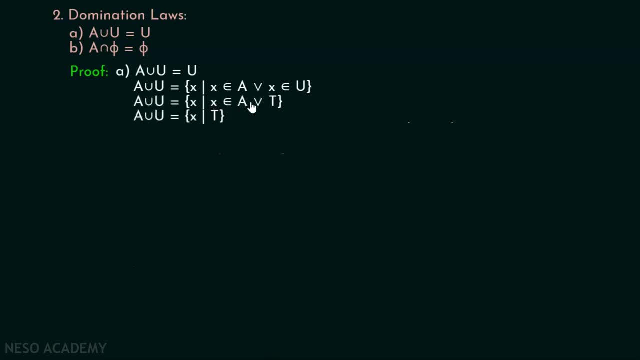 So we can replace this by capital T. And what is x belongs to A or true? We know that true or with anything is always true, Right, So we can replace this by T. This is how it looks like A union universal set is nothing but a set of all x such that true. 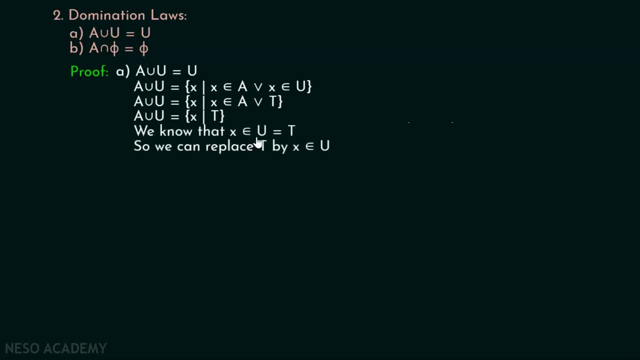 It doesn't make any sense at this moment. Right, We know that x belongs to universal set is true? Therefore, we can replace this capital T by x belongs to U. So let's replace this capital T by x belongs to U. 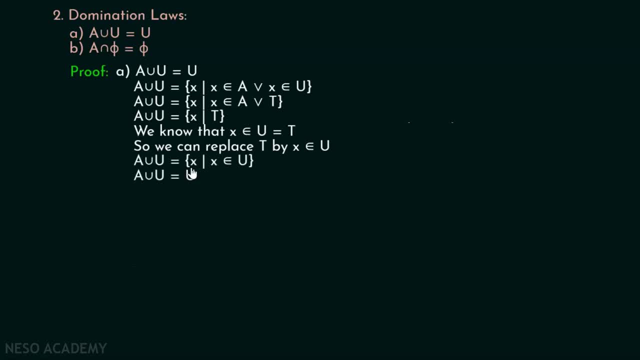 So what we are left with? We are left with this set, That is, set of all x, such that x belongs to U, Which means we are talking about universal set. Therefore, A union universal set is nothing but a universal set, Isn't that so? 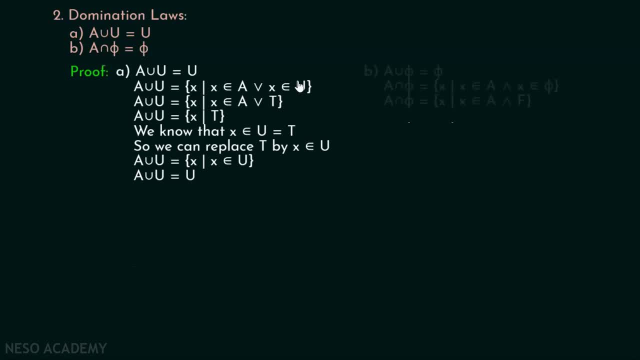 Now let's try to prove that A intersection phi is equal to phi. For this we will first write the definition of A intersection phi, which is nothing but a set of all x, such that x belongs to A and x belongs to phi. We know that x belongs to phi is false. 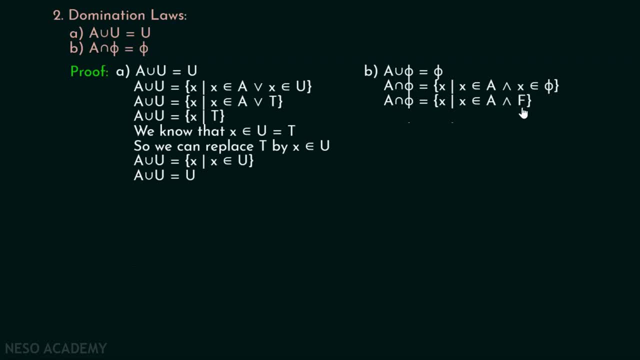 Therefore, we can easily replace this by F or capital F. Right, Here we know that false and with anything is always false, Right? Therefore, we can easily replace this whole statement by capital F. Again, it is not making any sense.